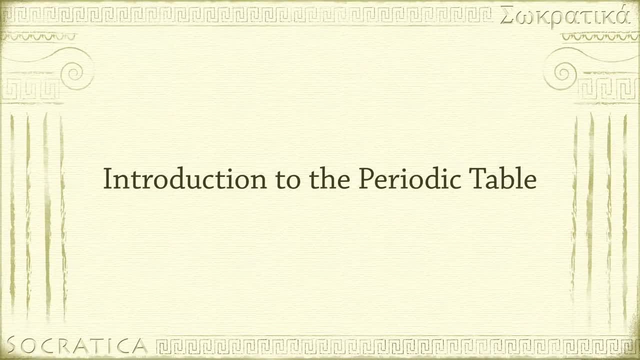 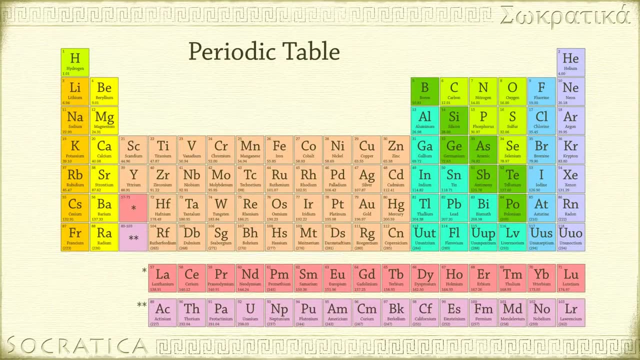 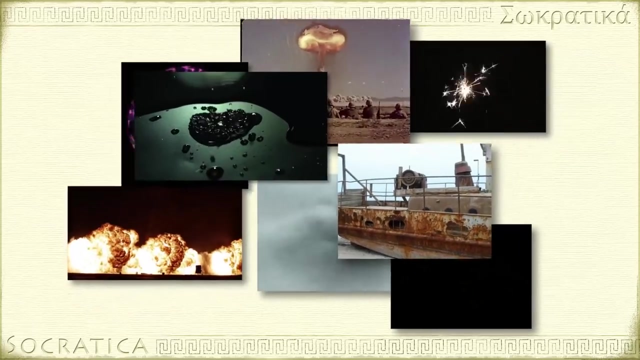 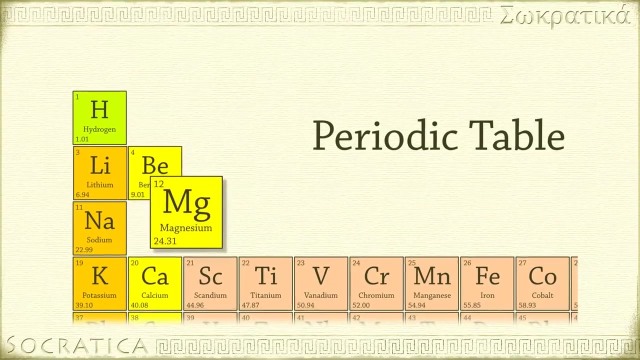 The Periodic Table is the most powerful tool chemists have for organizing chemical information. Without it, chemistry would be a chaotic, confusing jumble of seemingly random observations. What makes the Periodic Table really invaluable is its use as a predictive tool. You can predict. 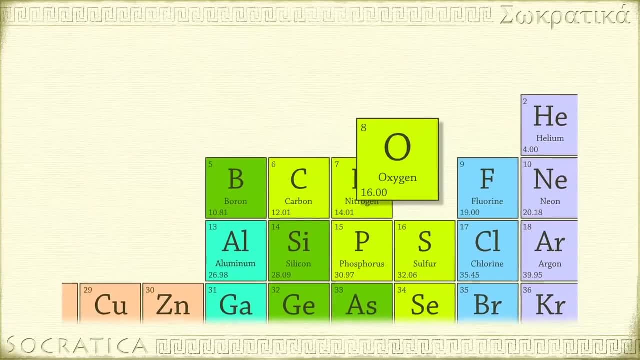 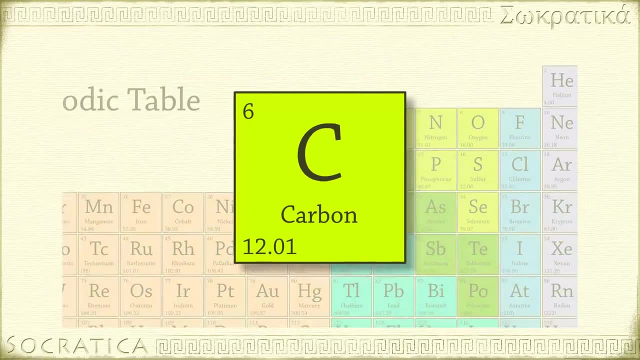 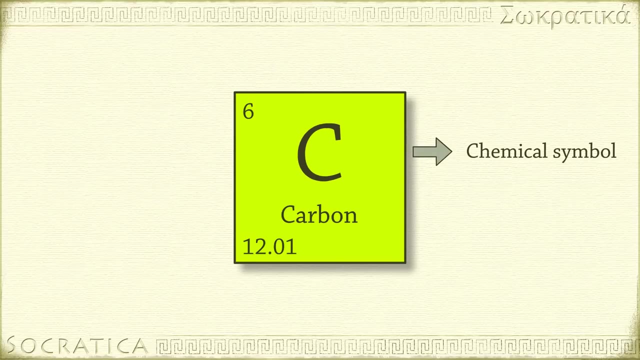 a lot about the chemical behavior of an element if you know where it is on the Periodic Table. Each element is represented by one square on the Periodic Table with a one or two-letter chemical symbol. Many of the chemical symbols are derived from the English name for the. 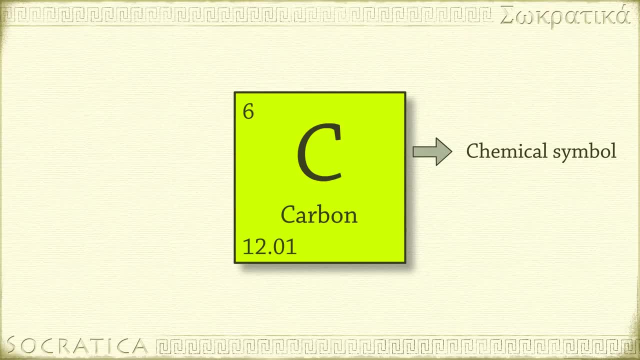 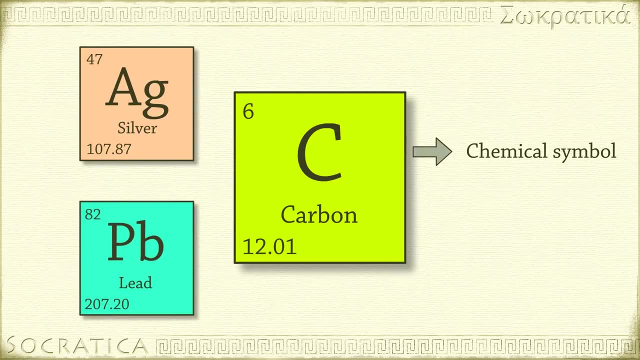 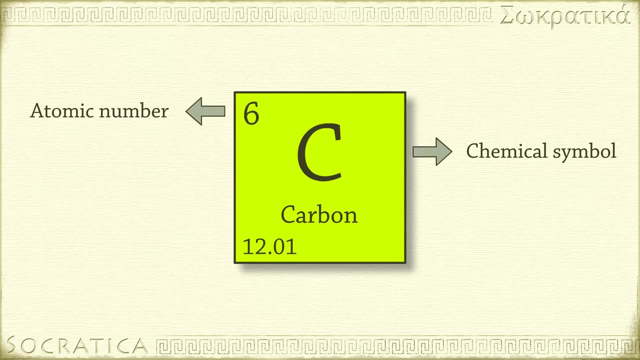 element, but some come from other languages. For example, the symbol for Silver is a- g. the symbol for Lead is p- b from the Latin Latin word plumbum. Above the chemical symbol is the atomic number of the element and below 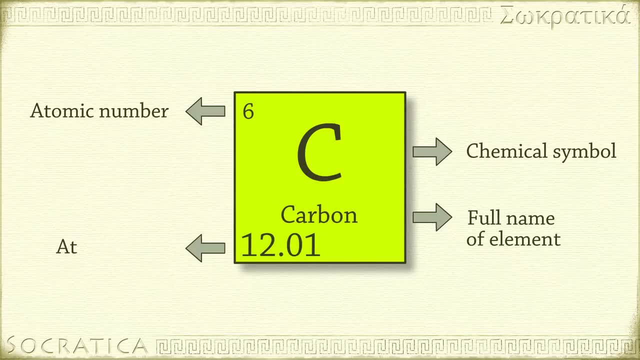 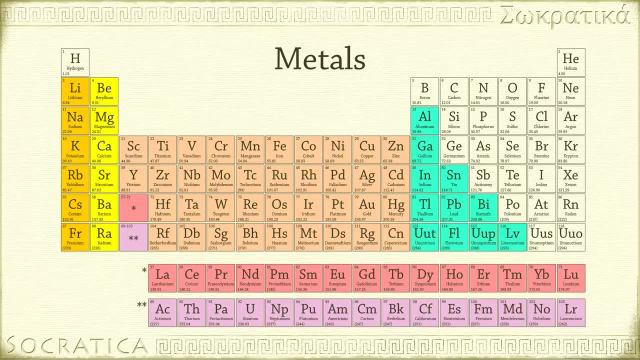 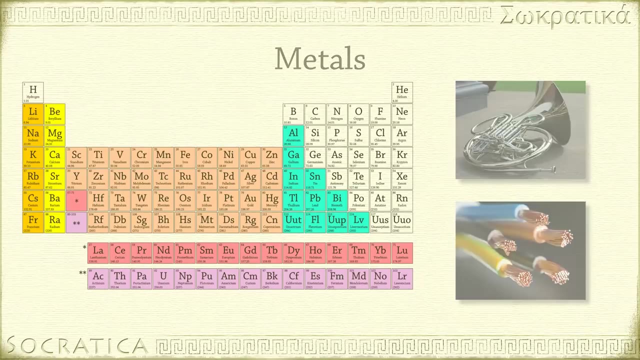 the symbol are the full name of the element and its atomic mass. Most elements are metals and you can find them on the left and in the middle of the periodic table. Metallic elements are typically shiny and are good conductors of heat and electricity. Non-metals are found. 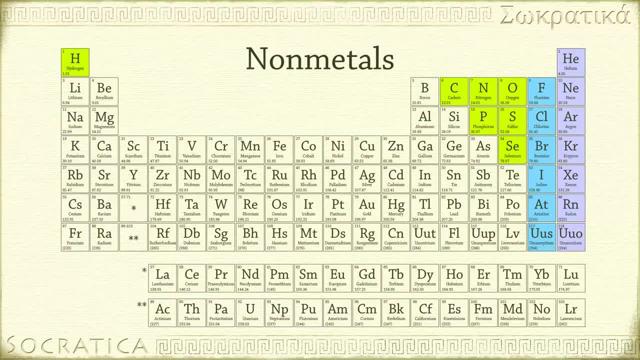 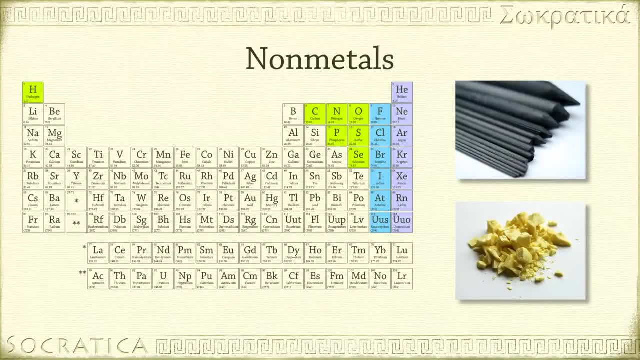 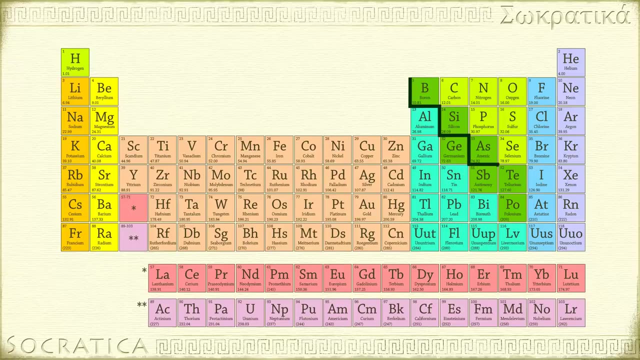 on the upper right of the periodic table. Except for hydrogen, there on the left it's also a non-metal. Non-metals generally are not shiny and are not good conductors of heat or electricity. The dividing line between metals and non-metals on the periodic table. 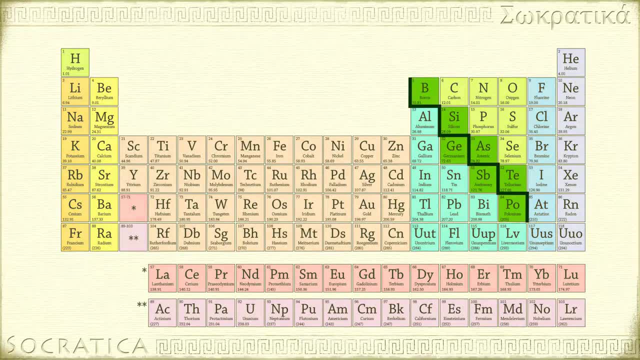 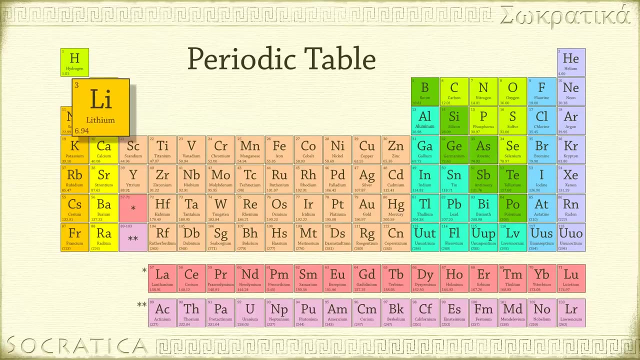 is drawn as a thick staircase. The elements that are found on either side of that staircase are often called metalloids, and they have properties that fall between metals and non-metals. Notice that the atoms are listed in order of increasing atomic number. as you read the 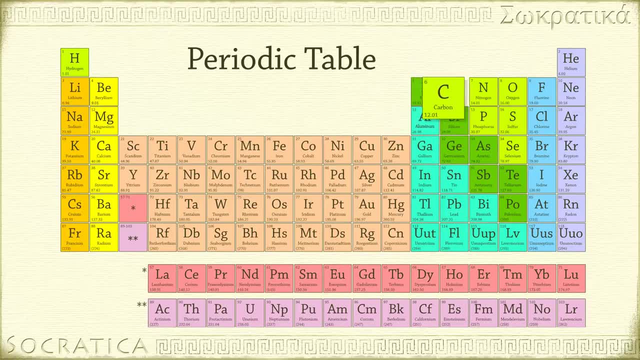 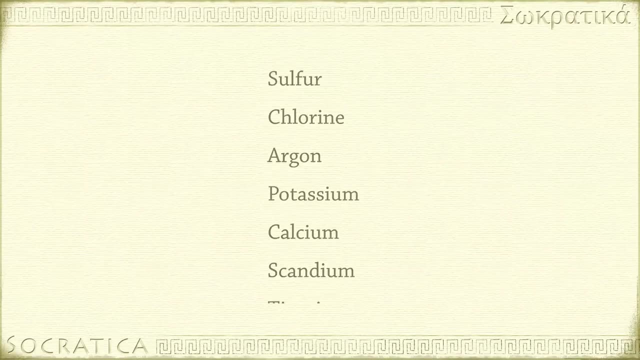 periodic table. from left to right, top to bottom, Each element has a unique atomic number, That's the number of protons in the nucleus of the atom. So why are the elements organized into rows and columns? Why don't we just put the elements in a long list? 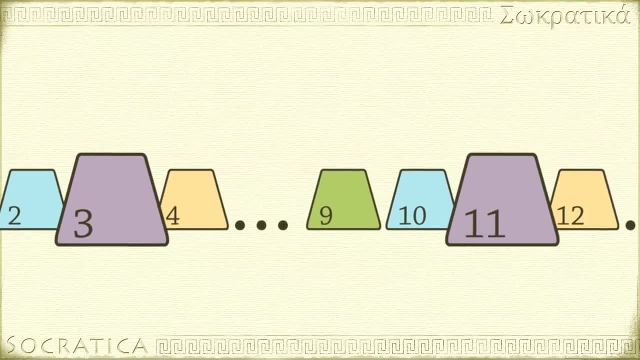 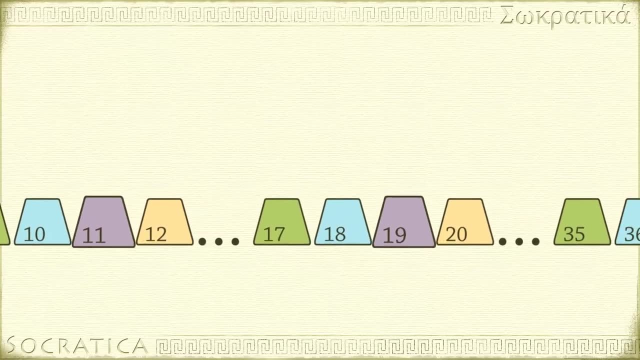 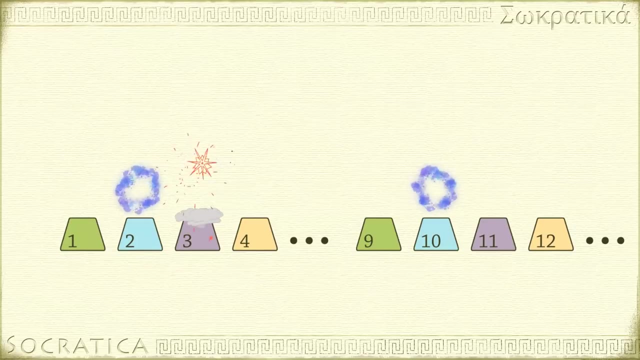 It turns out, if you arrange elements by atomic number, a pattern emerges. If you arrange, There is a periodicity or a repeating of certain characteristics. For example, every so often an inert gas appears. Right next to it will be an element that reacts violently with water. 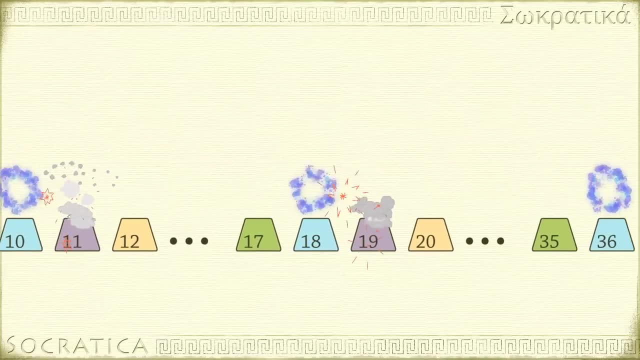 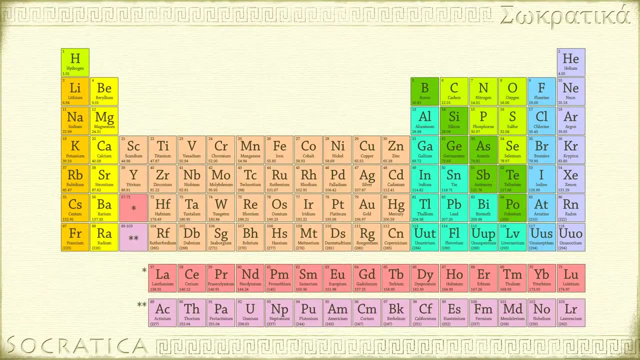 This periodic repetition is known as the periodic law. This is the basis for organizing the elements in the periodic table into columns. A vertical column of elements is called a group or a family. The elements in a group have similar chemical properties. We now know that's because they have similar valence electron configurations. 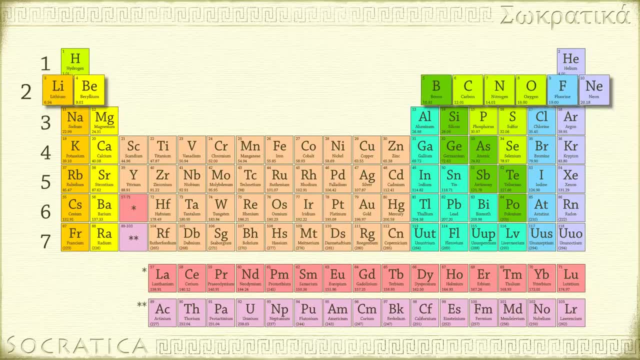 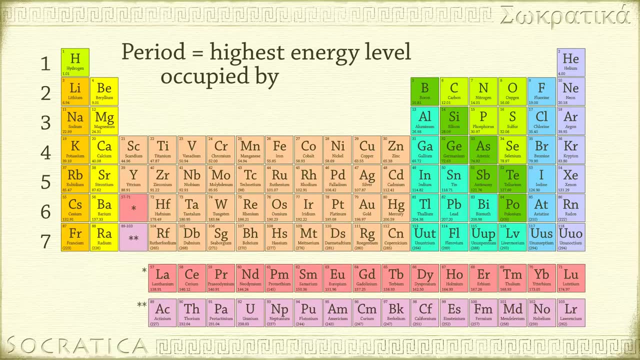 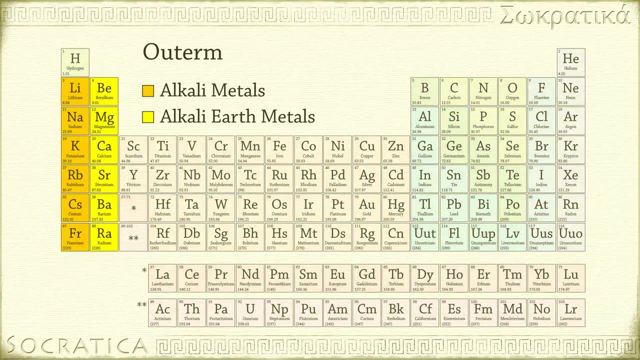 There are seven horizontal rows in the periodic table. These rows are called periods. Each row corresponds to a different energy level occupied by electrons. The two groups on the left are the alkali metals and the alkali earth metals, The s orbitals in the outermost shell. 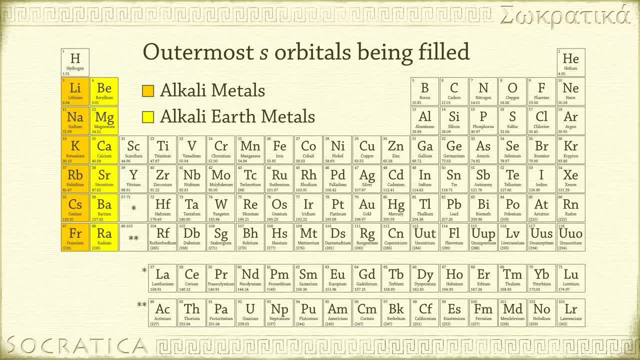 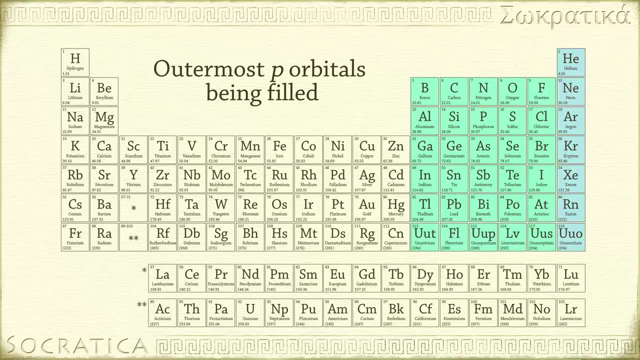 of the atom are being filled in these groups. On the right is a block of six columns. These elements have the outermost p orbitals being filled. Notice. on the far right are the noble gases which all have a filled valence shell of electrons. 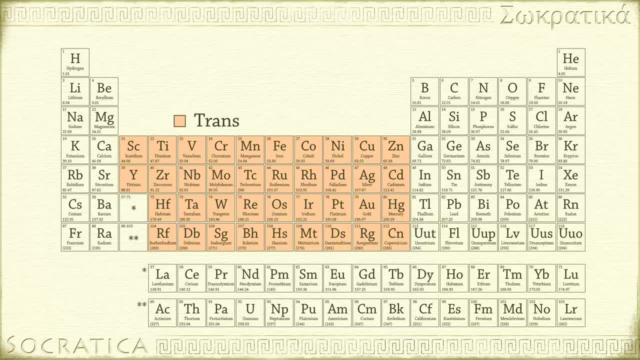 In the middle is a block of ten columns, the transition metals. In these elements, the outermost d orbitals are being filled. The asterisks take you to the bottom of the periodic table, where there are two rows of fourteen columns. These are the inner transition metals. 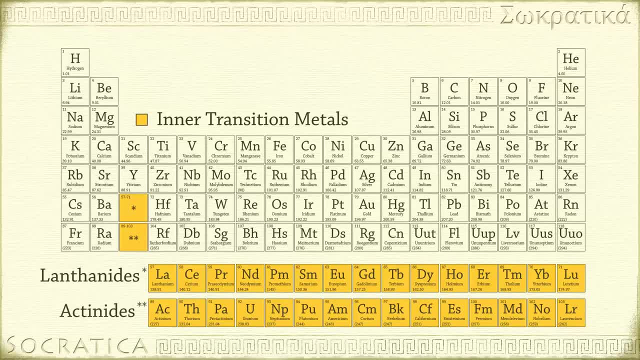 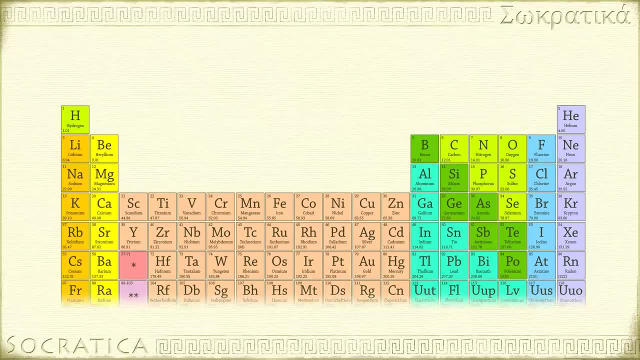 also known as the lanthanides and actinides. These elements have the outermost f orbitals being filled. The groups in the periodic table have been numbered in a variety of ways over the years, Depending on which periodic table you look at. 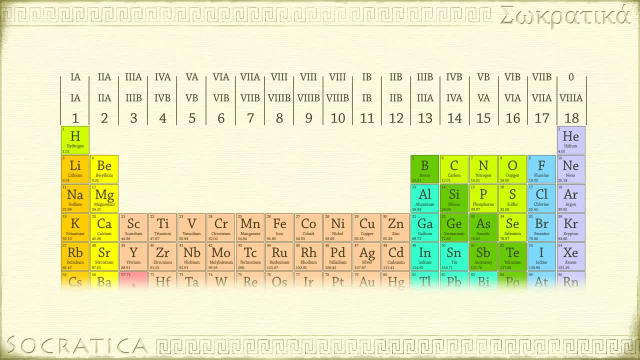 it may have one, two or even three different systems for numbering the groups. There are many groups labeled with Roman numerals and a's and b's. This system was popular in North America and Europe. Unfortunately, the designations were somewhat arbitrary. 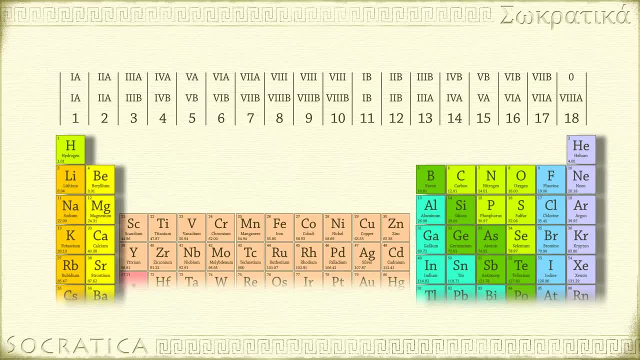 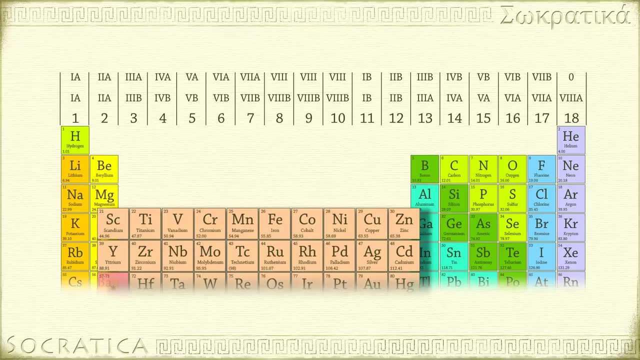 In North America, the a groups were the s and p blocks, known as the representative elements, and the b groups were the d block, the transition metals. Meanwhile, in Europe, the a groups were on the left and the b groups were on the right. 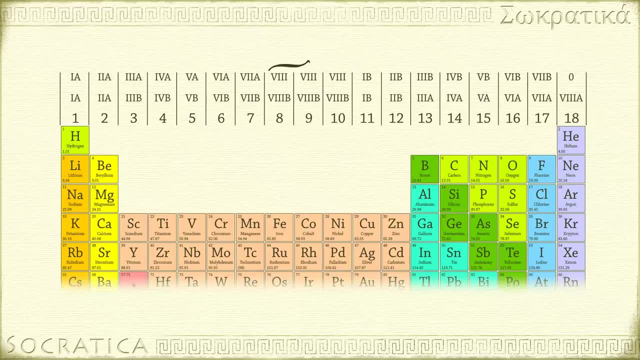 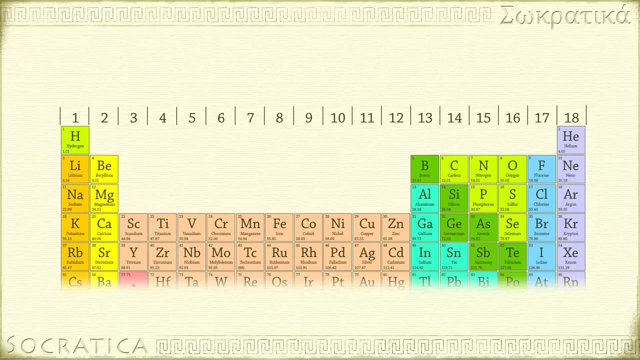 And in both systems there was one triple-sized group called Roman numeral VIII. To eliminate all this confusion, the International Union of Pure and Applied Chemistry proposed a system that numbers the groups I through XVIII, with no a's or b's. This is an example of the sorts of refinements 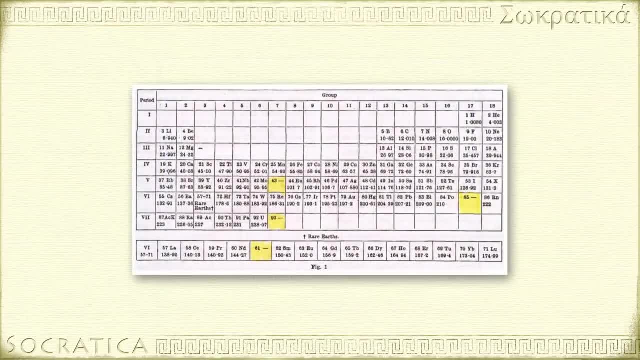 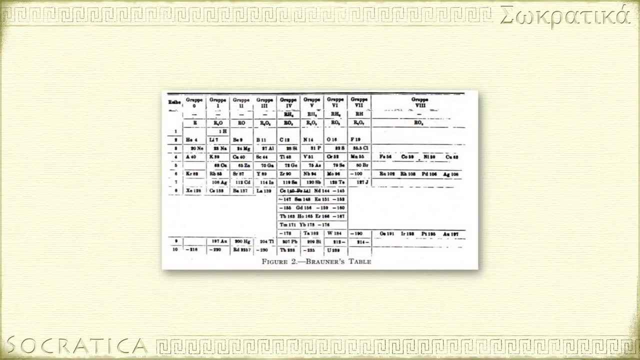 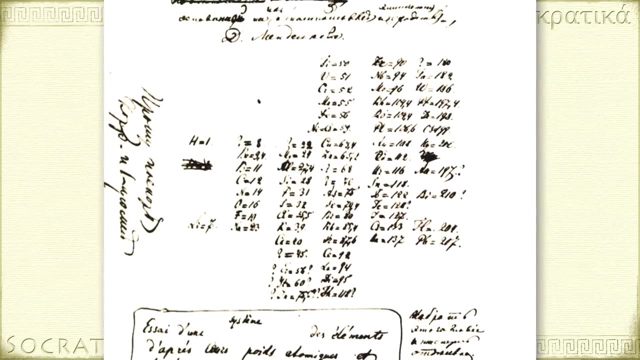 that have changed the periodic table gradually over the years as new discoveries were made and chemists came to agree with the experiments about how to present the new information. You may not even recognize the first periodic table. Fewer than 70 elements had been discovered in the mid-1800s. 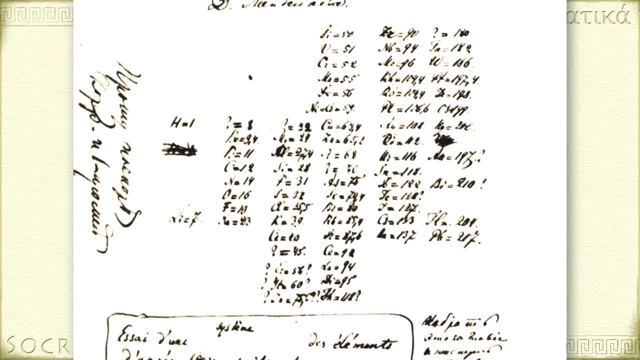 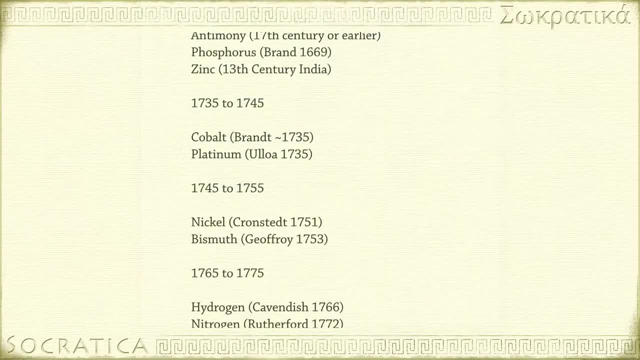 They didn't know about noble gases yet At that point there was no agreed-upon way to list the elements that was of any help to chemists. For example, listing them in the order of discovery didn't tell you anything about their chemical behavior. 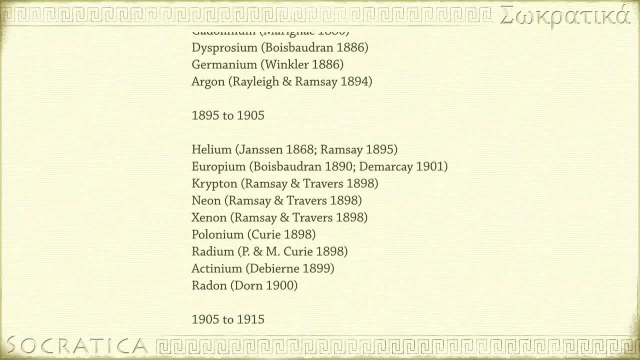 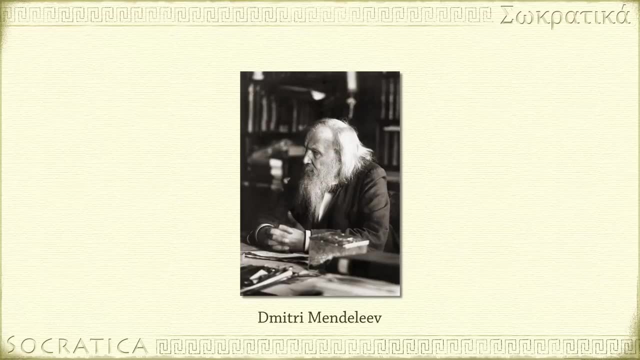 so that kind of list would be useless if you didn't have any kind of predictive tool. This was the state of affairs when Russian chemist Dmitri Mendeleev developed the periodic table In 1869, Mendeleev came up with the idea. 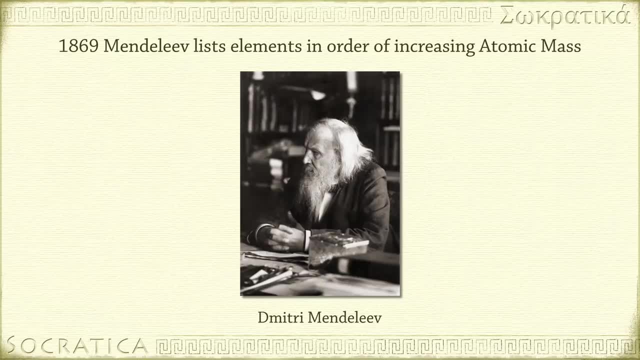 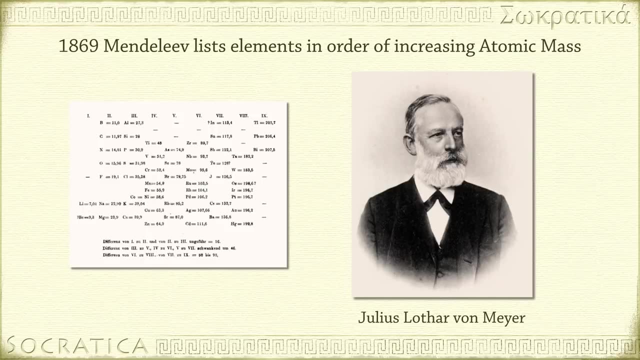 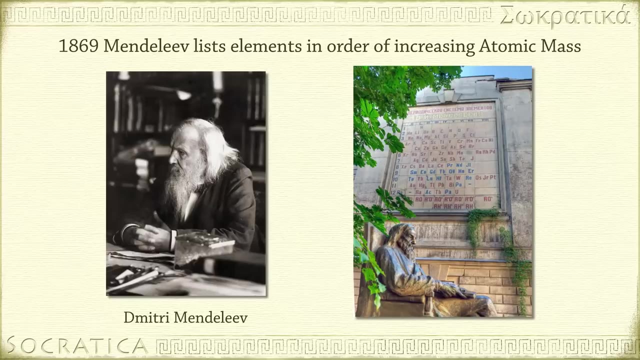 of listing the elements in order of increasing atomic mass. Almost simultaneously, Lothar Meyer in Germany published a nearly identical system for classifying elements. We generally give credit for the discovery to Mendeleev because he devoted so much time and effort championing this new system. 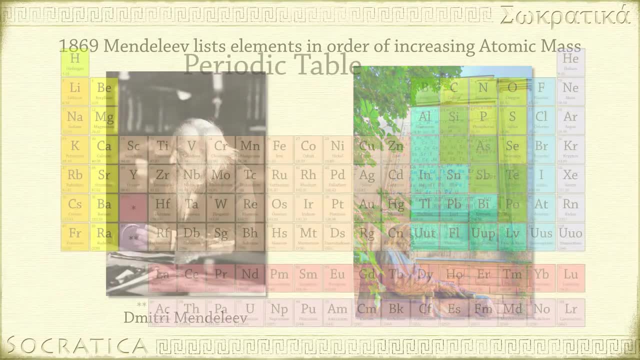 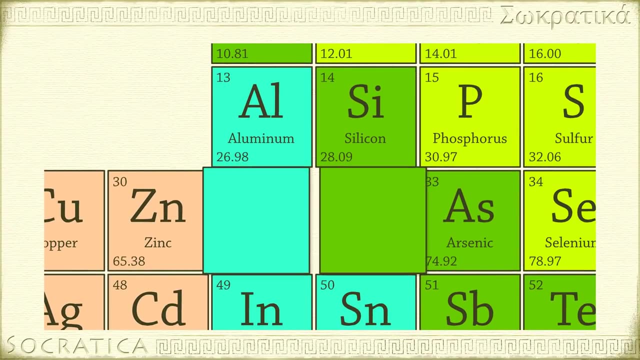 and he helped it become widely accepted. Mendeleev insisted that elements with similar properties be listed together, and because of this there were gaps in his table. Mendeleev boldly proposed the existence of a number of elements that had not yet been found that would one day fill in these gaps. 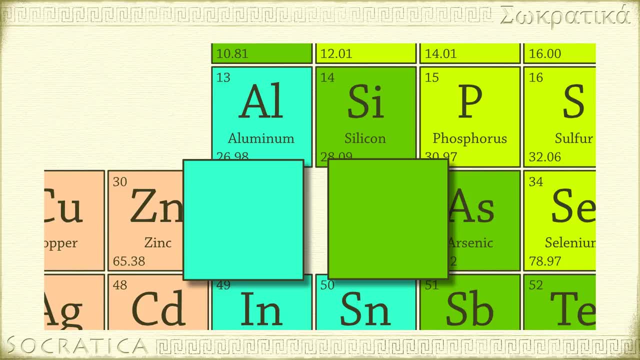 He named them for their positions in his table. For example, the proposed element eka-aluminum would reside under aluminum and eka-silica would go under silicon. Some years later these elements were indeed found and their characteristics closely matched Mendeleev's predictions.